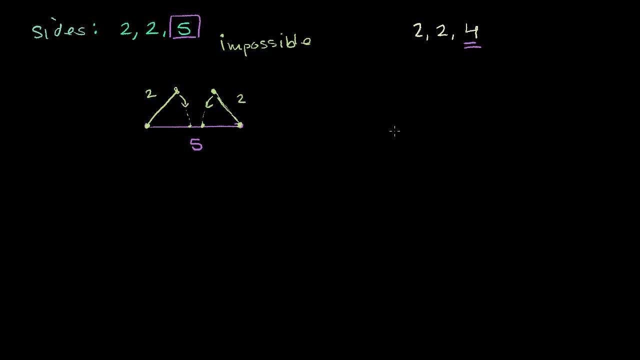 So let's draw the side of length 4.. Let me draw it a little bit shorter. So that's your side of length 4.. And then, in order to make the two sides of length 2 touch, you have to rotate them all the way inward. 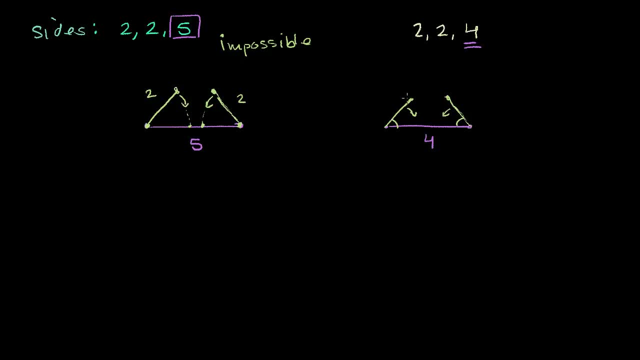 so that both this angle and this angle essentially have to become 0 degrees. And so your resulting triangle: if you rotate this one all the way in and you rotate this one all the way in, the points will actually touch, But this triangle will have no area anymore. 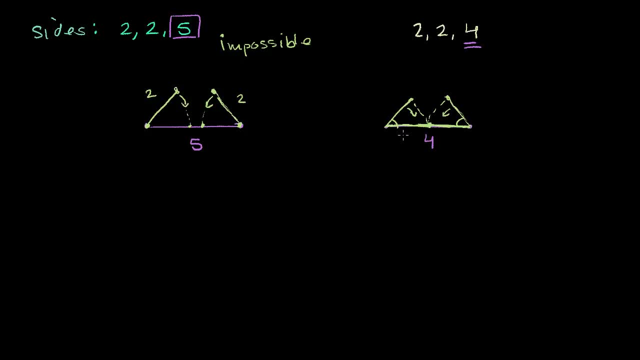 This will become a degenerate triangle And it really looks more like a line segment. Let me write that down: This is a degenerate. In order for you to draw a non-degenerate triangle, the sum of the other two sides have to be longer than the longest side. 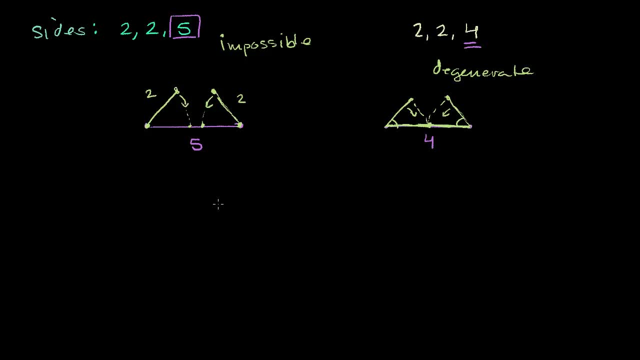 So, for example, you could definitely draw a triangle with sides of length 3,, 3, and 5.. So that's the side of length 5. And then if you were to rotate all the way in those two points would, if you were to rotate all the way in. 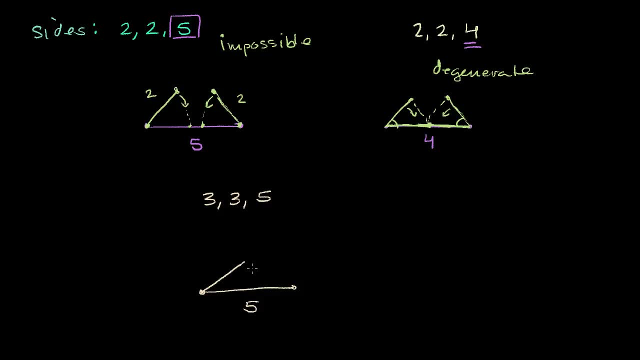 rotate. Let me draw this a little bit neater. So let's say that's where they connect. And we know that we could do that because if you think about it, if you were to keep rotating these, they're going to have to pass each other at some point. 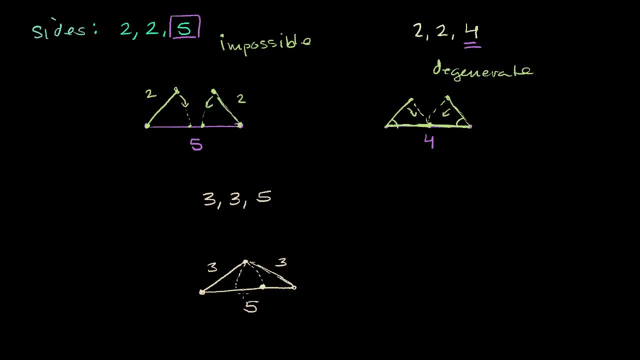 They're going to have to overlap. If you tried to make a degenerate triangle, these points wouldn't touch. They'd actually overlap by one unit right over here. So you could rotate them out and actually form a non-degenerate triangle. So this one you absolutely could. 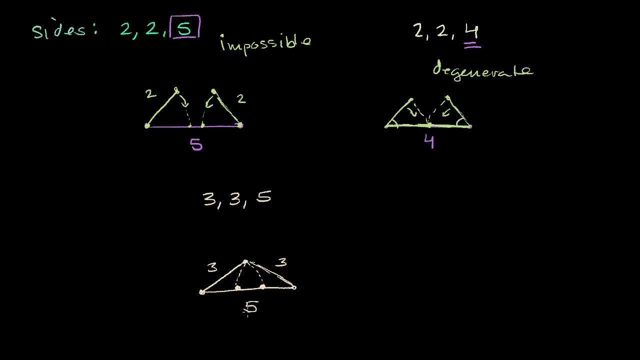 And then there's another interesting question: Is this the only triangle that you could construct That has sides of length 3,, 3, and 5?? Well, you can't change this length, So you can't change that point and that point. 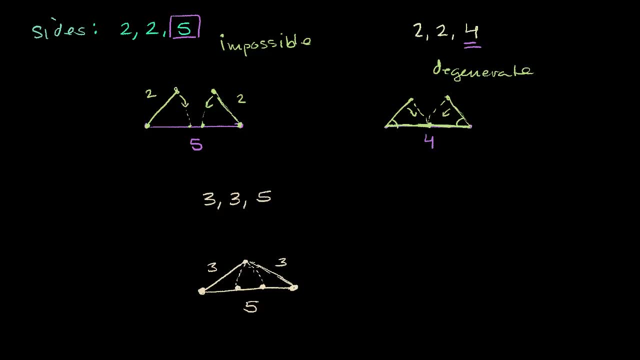 And then you can't change these two lengths, So the only place where they will be able to touch each other is going to be right over there. So this right over here is the only triangle that meets those constraints. You could rotate it and whatever else. 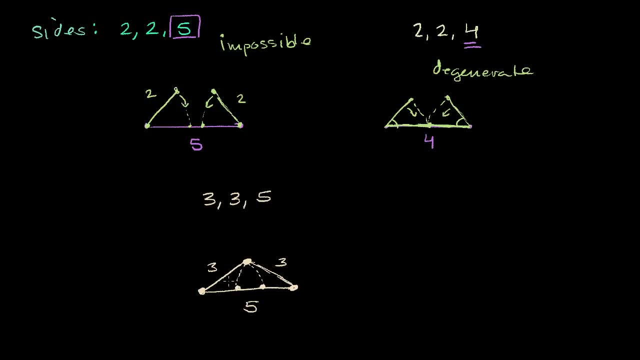 but if you rotate this, it's still the same triangle. This is the only triangle that has sides of length 3,, 3, and 5. You can't change any of the angles somehow to get a different triangle. OK, OK. All right.